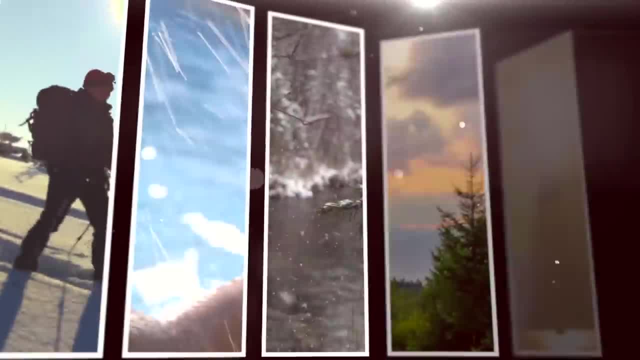 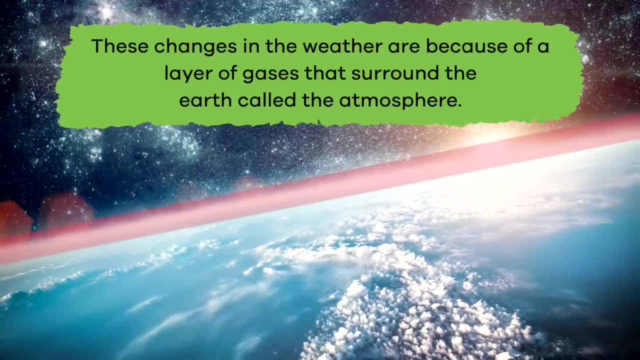 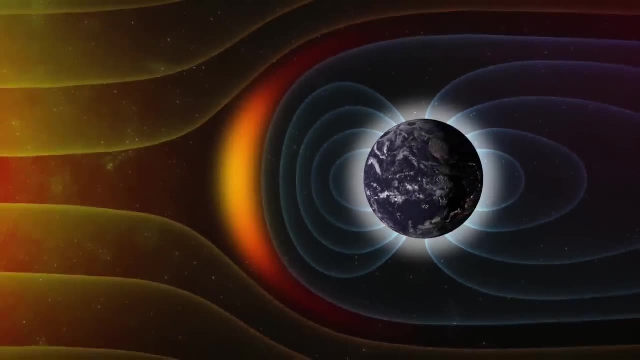 or cold. Most of the time, it is at least a few of these things all at once. These changes in weather are because of a layer of gases that surround the Earth called the atmosphere. The atmosphere also acts as a shield, protecting life and helping keep. 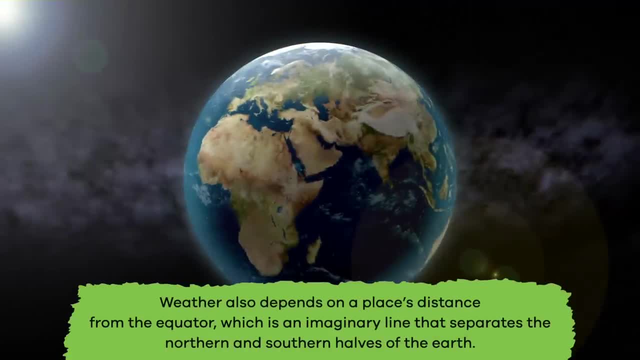 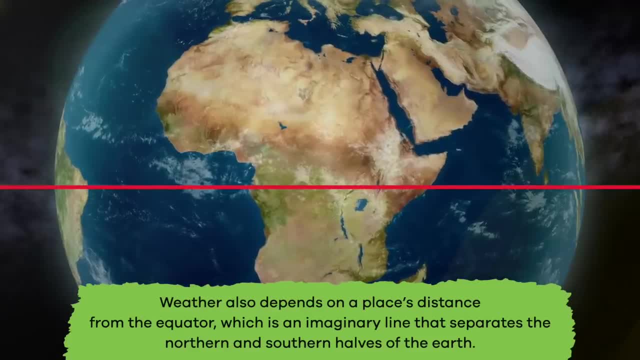 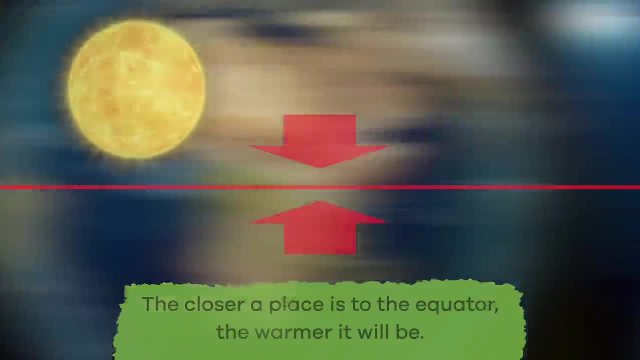 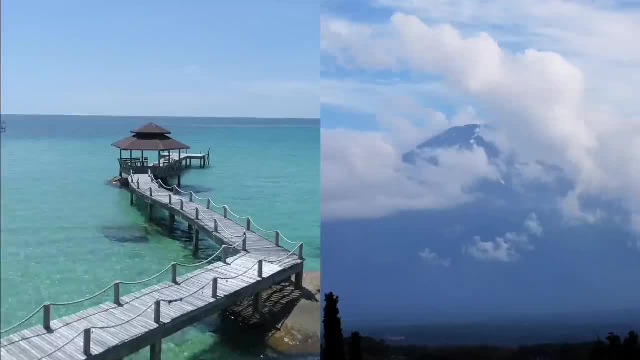 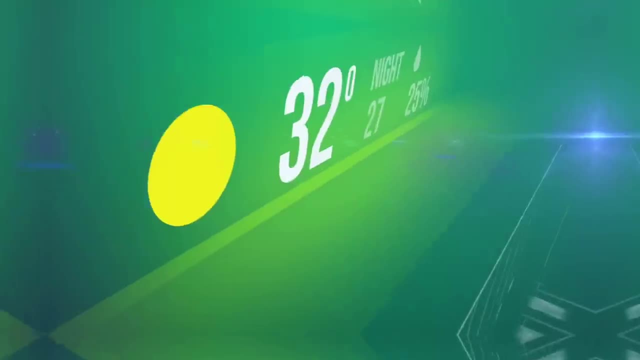 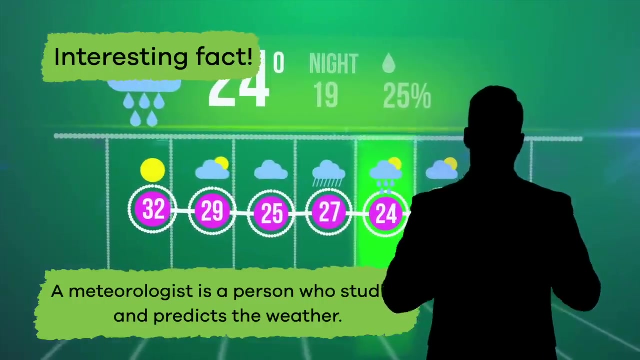 weather. you will see, For example, the weather near the ocean is often a lot different than the weather near a tall mountain range. Here is an interesting fact: A meteorologist is a person who studies and predicts the weather. You might have even seen a meteorologist sometime. 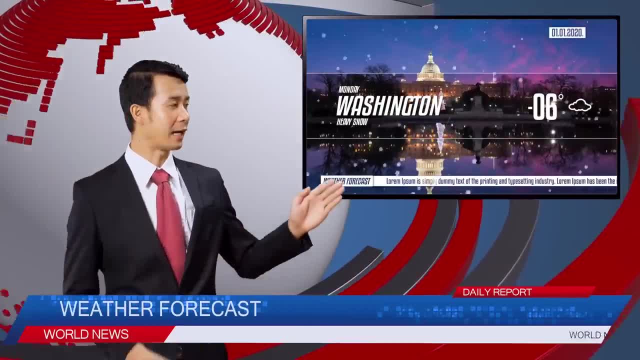 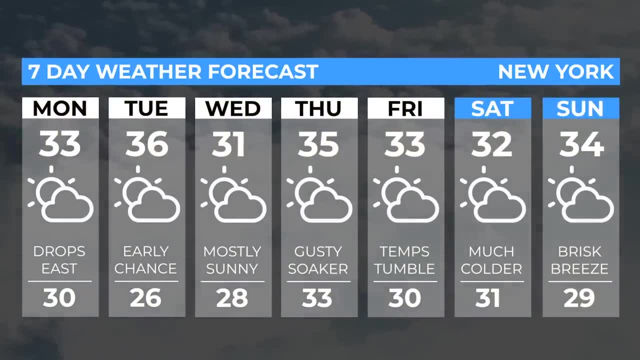 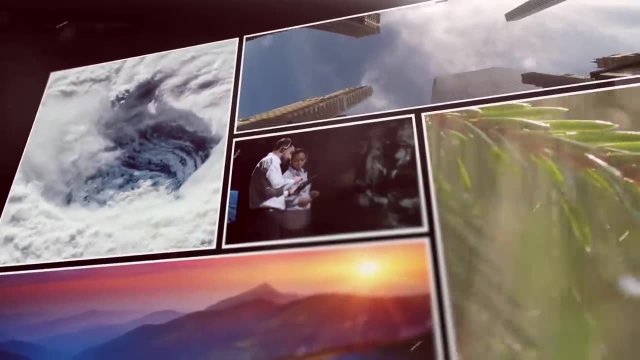 on the news. They are the people who stand in front of a weather map and give forecasts, or educated predictions, of what the weather will be like during the week in the area where you live. Cool, right Now that we have talked about what weather is, let's talk about the different types of weather. 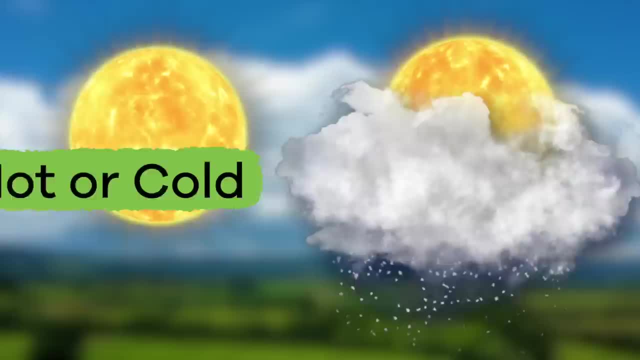 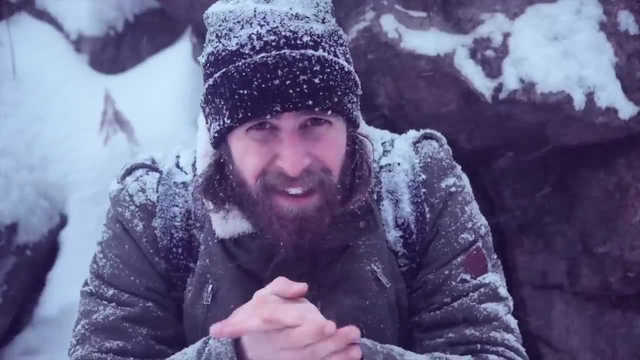 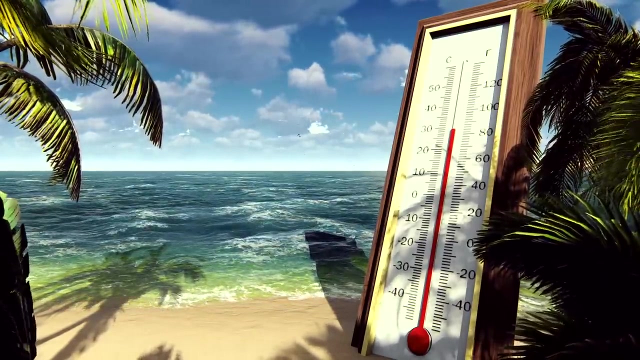 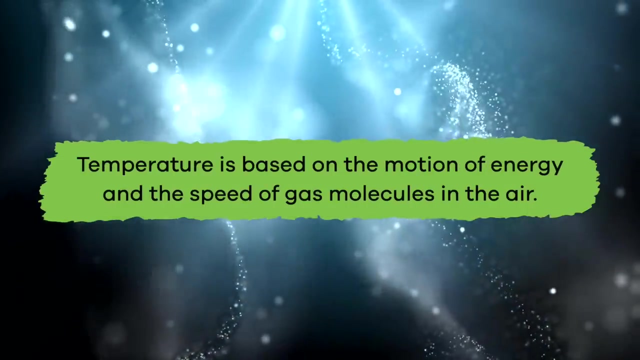 and how the weather will be different. First off, weather can be hot or cold, or somewhere in between. The way that this hotness or coldness is measured is by temperature. Temperature is based on the motion of energy and the speed of gas molecules in the air. If the gas molecules are moving faster, the temperature will 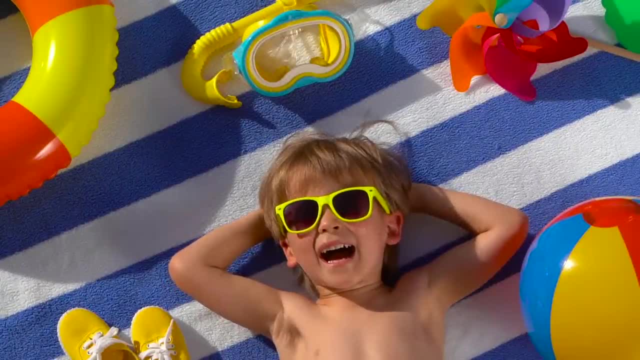 get faster. If the gas molecules are moving faster, the temperature will get faster. If the gas molecules are moving faster, the temperature will get faster. If the gas molecules are moving faster, they will get higher, meaning that the weather gets hotter. 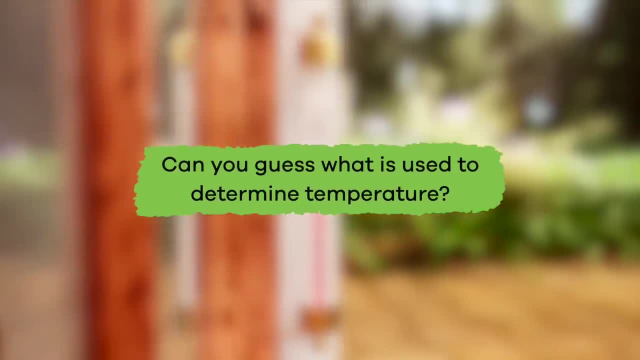 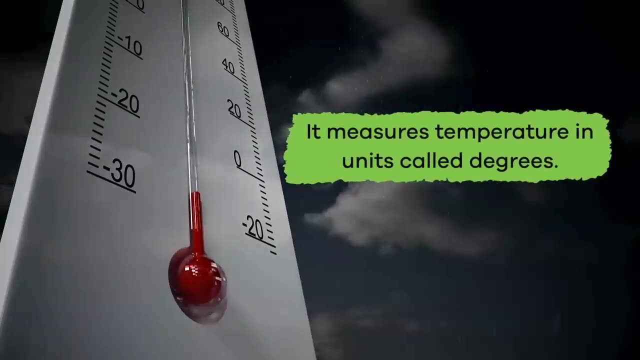 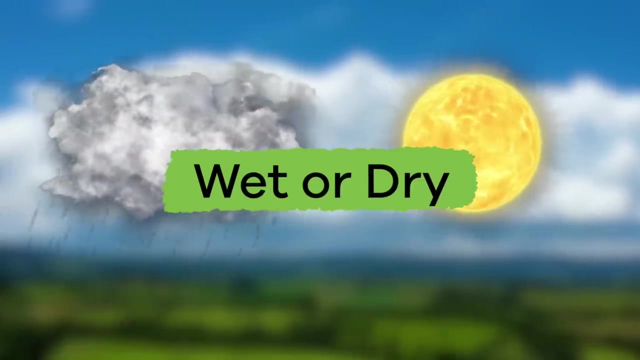 Can you guess what is used to determine temperature? That is right. It is a tool called a thermometer. it measures temperature in units called degrees, Wet or Dry. Have you ever been near the ocean? What about deserts? The most dry land at the sea is mets Today- apparently wet. Steve. sometime inGenuchesk is up on fire. 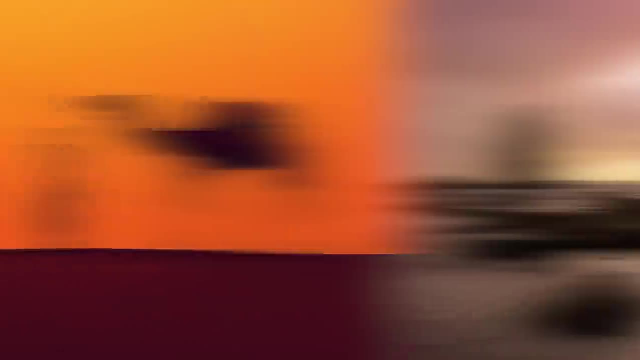 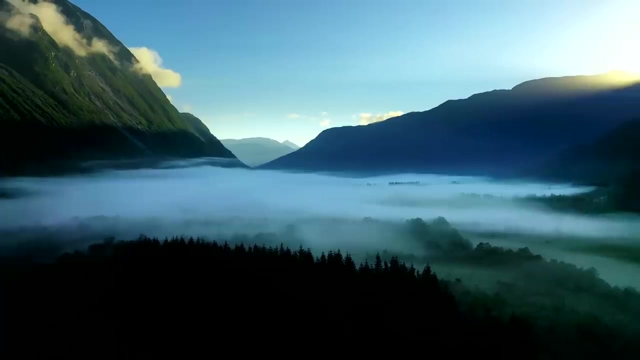 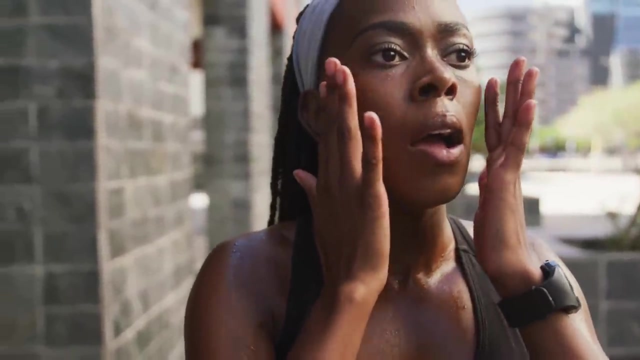 air around you can feel different depending on where you are in the world. This difference is called humidity, which tells us the amount of water vapor in the air. Even though you cannot see this water, you can definitely feel it. The higher the humidity, the more moisture. 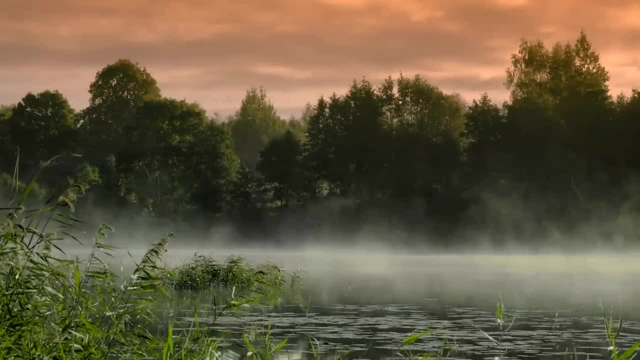 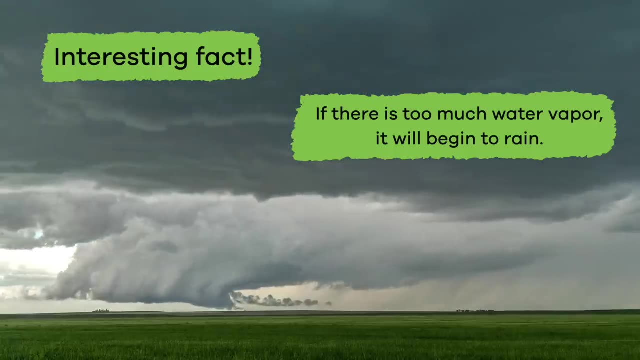 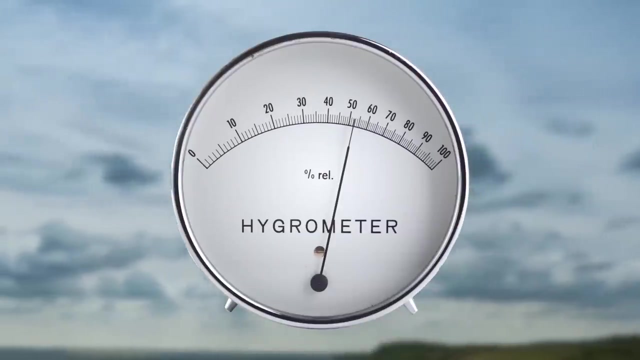 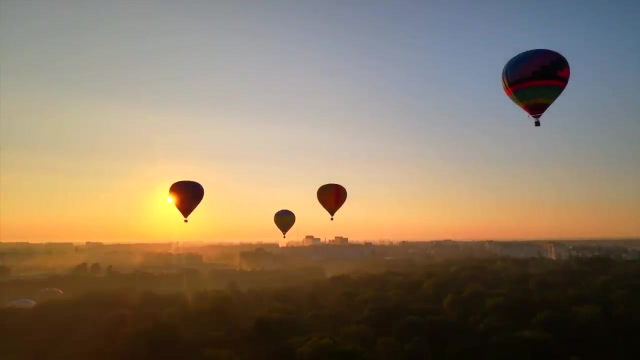 or water vapor there is in the air. Here is another interesting fact: If there is too much water vapor, it will begin to rain. Humidity is measured by a tool called a hygrometer. Clear or cloudy? Did you know that air pressure affects whether or not it is a clear or cloudy day? 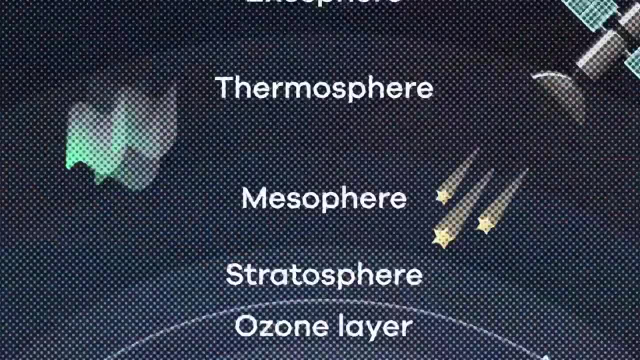 Remember when we talked about the air pressure. It is a clear or cloudy day. Remember when we talked about the air pressure. It is a clear or cloudy day. Remember when we talked about the atmosphere? Well, air pressure is the weight of the atmosphere pressing down on the earth. 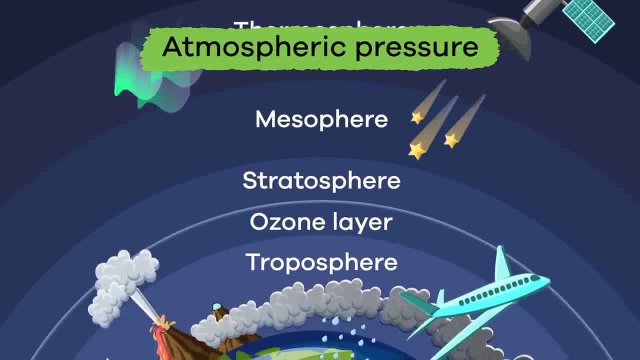 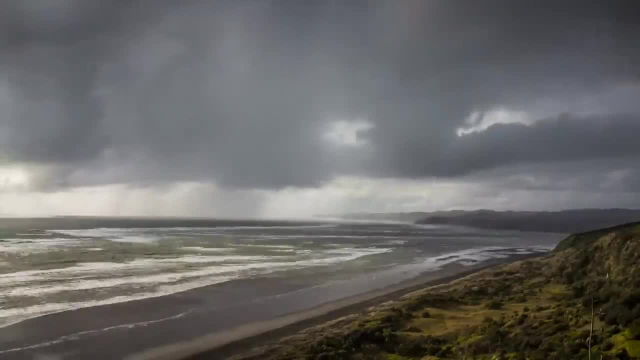 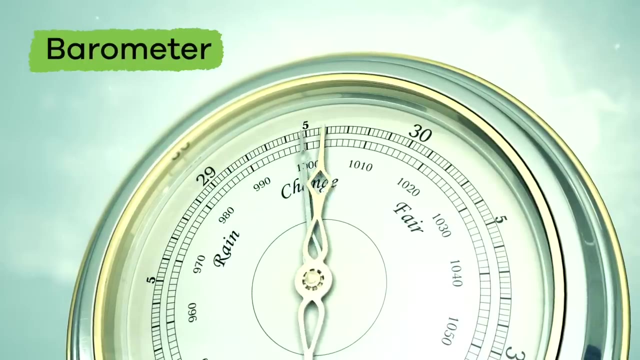 which is why it is also sometimes called atmospheric pressure. Like our old friend humidity, air pressure affects all parts of the weather each day. How is air pressure measured, you ask? By a tool called a barometer. There are two types of air pressure: high. 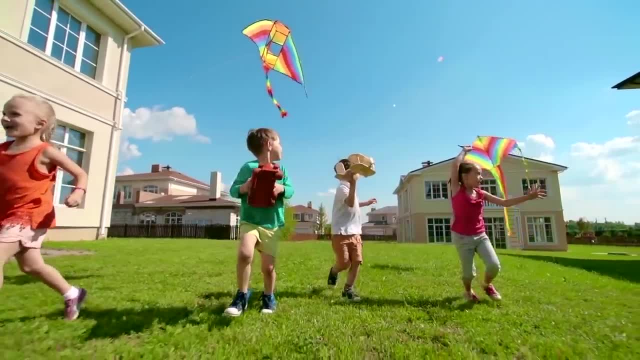 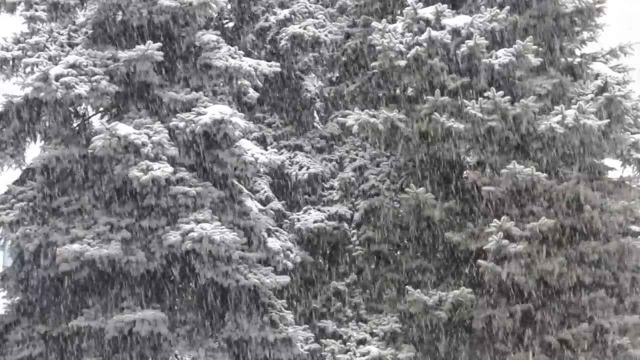 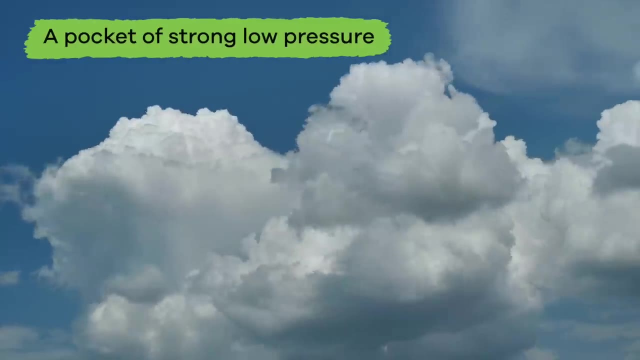 and low High pressure usually means that the weather will be fair and sunny. Low pressure, on the other hand, brings clouds, rain or snow. Have you ever wondered what causes thunderstorms? A pocket of strong low pressure. You can literally feel it in the air. 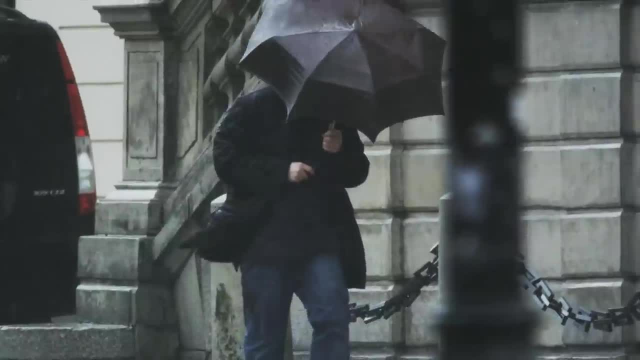 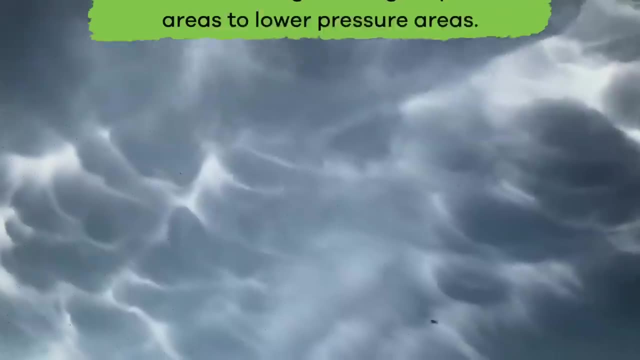 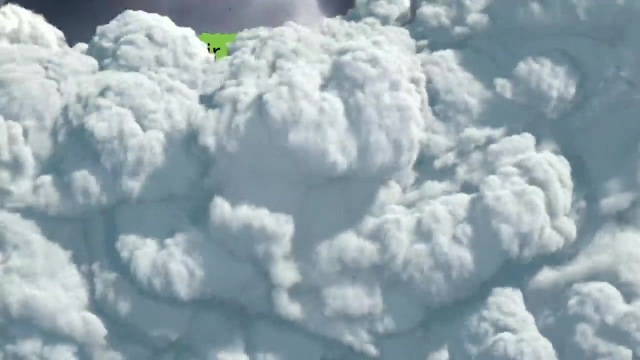 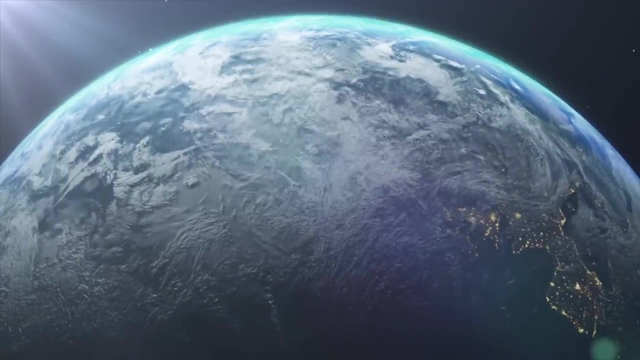 Calm or stormy. When you find yourself stuck in a storm, you might notice that wind is almost always involved. Wind is air moving from higher pressure areas to lower pressure areas. Wind speed is also affected by the heating of the earth's surface and the rotation of the earth. The speed of wind can also be changed by the landforms around it- Stuff like mountains, bodies of water and vegetation, which is why sometimes wind can start as a gentle breeze and then change into a super strong gust. The airspeed of wind is measured by a device called. 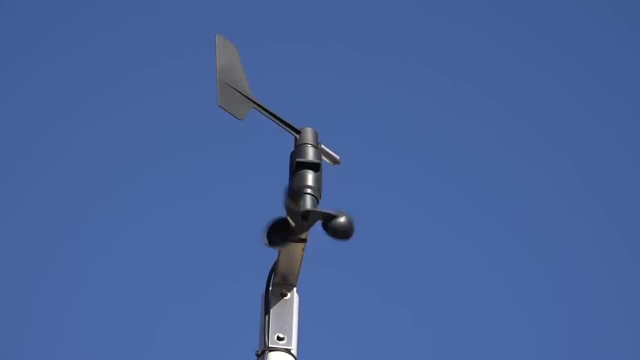 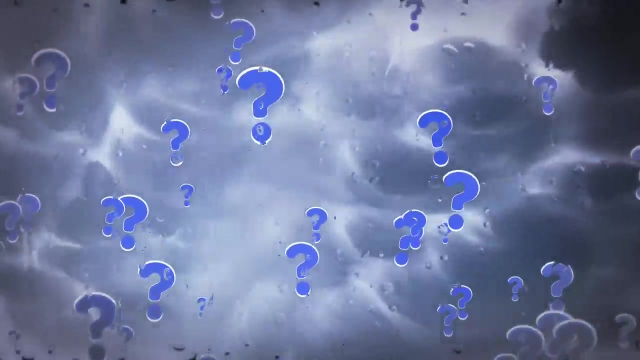 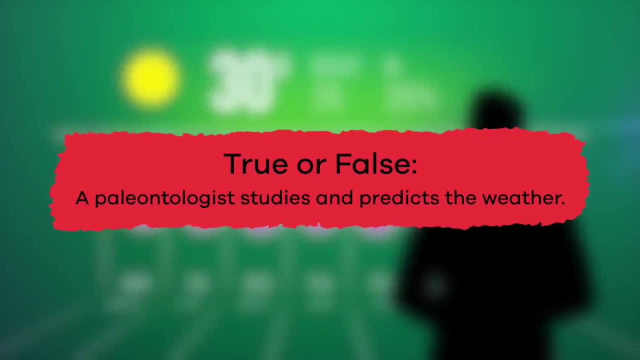 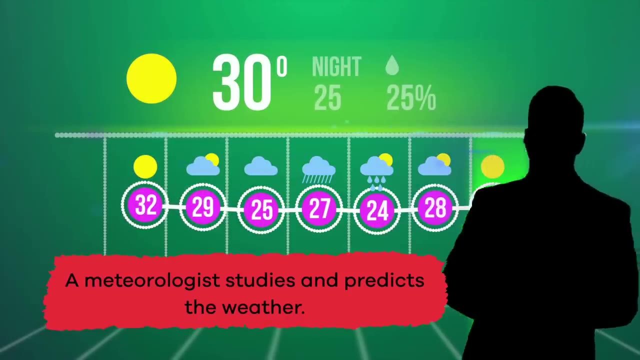 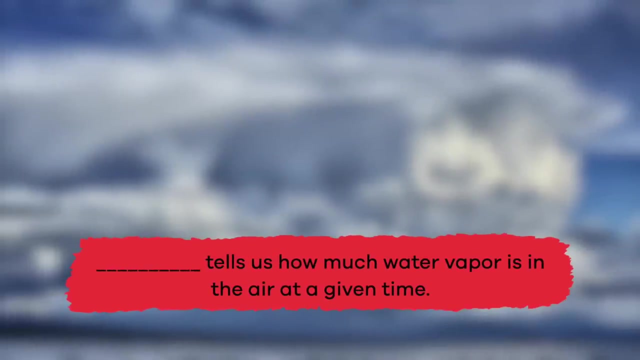 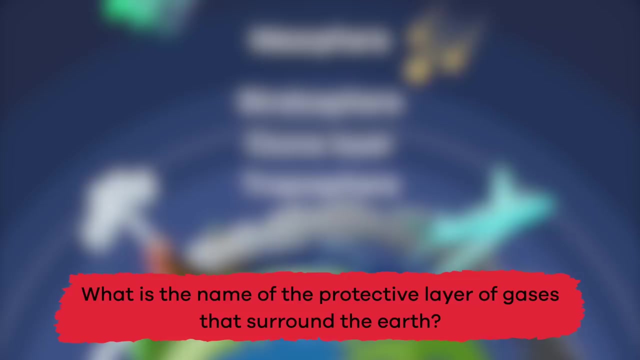 False A- paleontologist studies and predicts the weather. False A- meteorologist studies and predicts the weather A paleontologist studies. fossils- Fill in the blank. Blank tells us how much water vapor is in the air at a given time. B- What is the name of the protective layer of gases that surround the Earth? 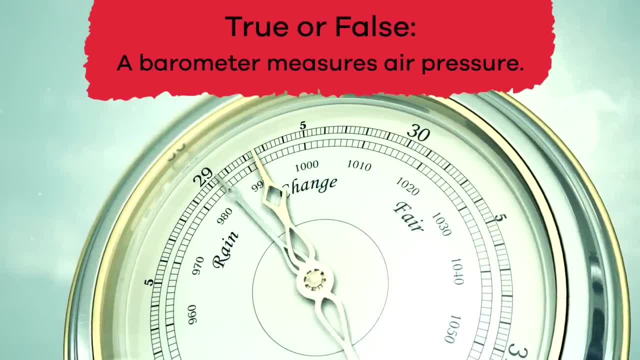 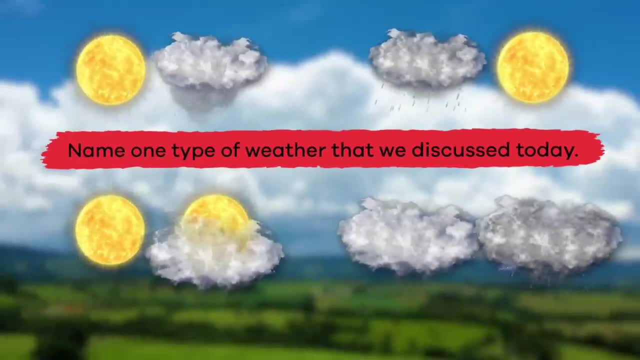 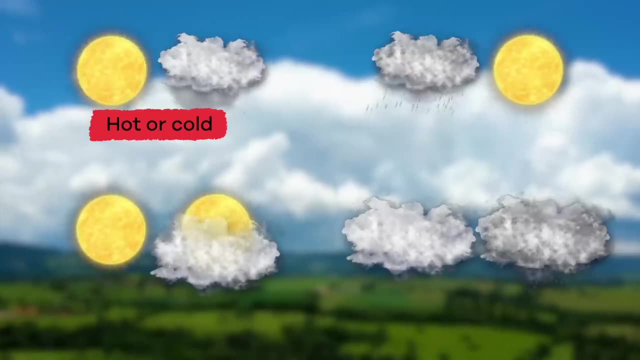 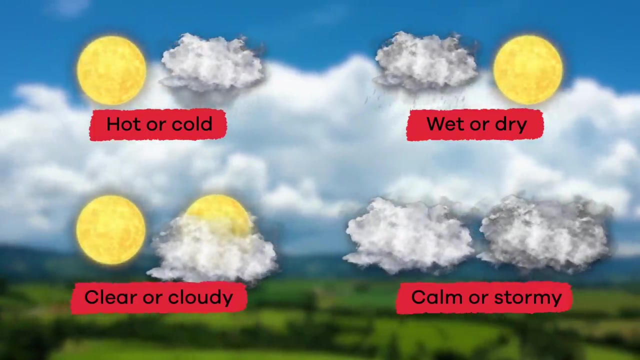 The atmosphere, True or false? A barometer measures air pressure. True Name, one type of weather that we discussed today. You're right: Hot or cold, Wet or dry, Clear or clear, Cloudy or calm or stormy. Nice job, weather wonders. 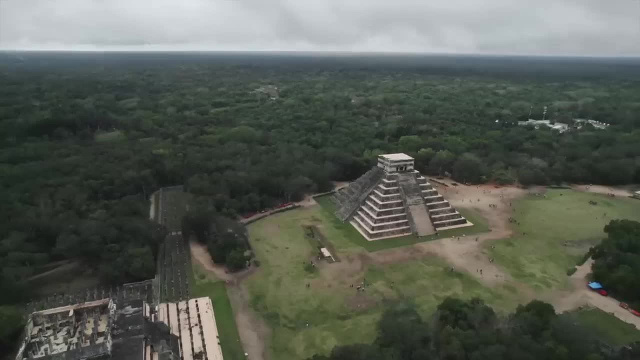 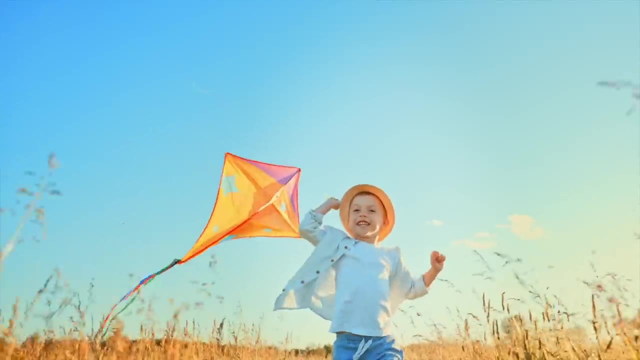 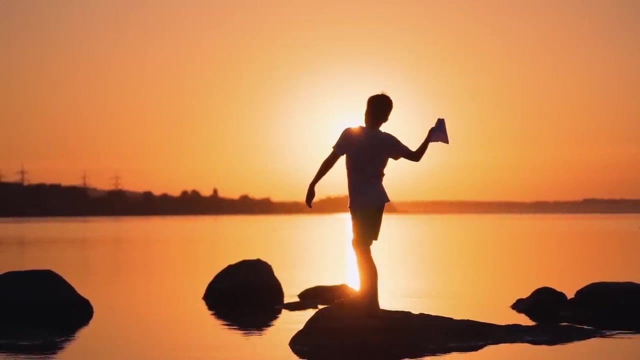 No matter if you live near the equator or on top of a tall mountain, you will always be surrounded by weather. The next time you are outside, try to see if you can figure out exactly what the weather is like using all the information you have learned today. 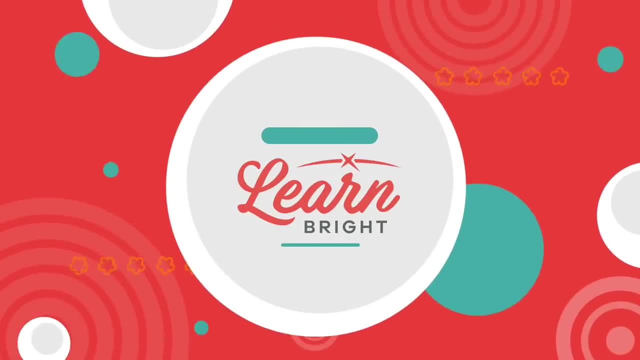 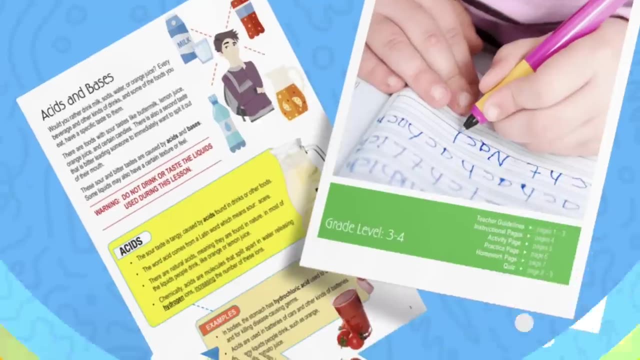 Thanks for watching. See you next time. Hope you had fun learning with us. Visit us at LearnBrightorg for thousands of free resources and turnkey solutions for teachers and homeschoolers.